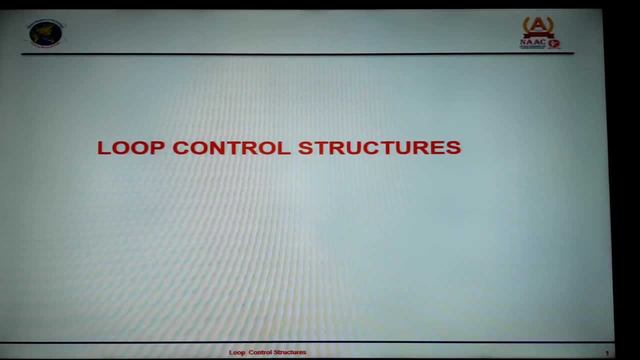 But then tomorrow somebody else may come and say I want to drink 10 times. Then probably as a programmer, I land up doing, you know, enhancing the number of lines in the if statement and then now make it 10 printer statements drinking coffee. When I look at that particular aspect of human being, you know, basically human beings are considered to be the most greediest fellow on this earth And definitely I'm sure this will not solve the purpose. 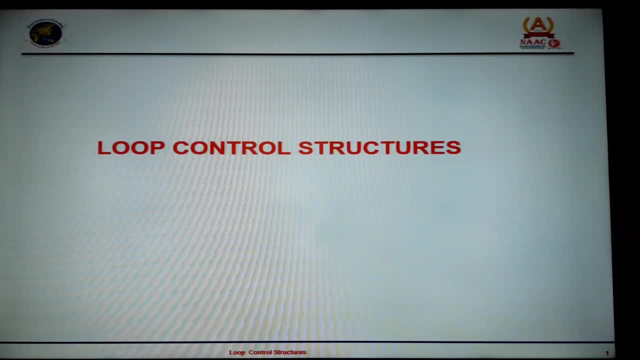 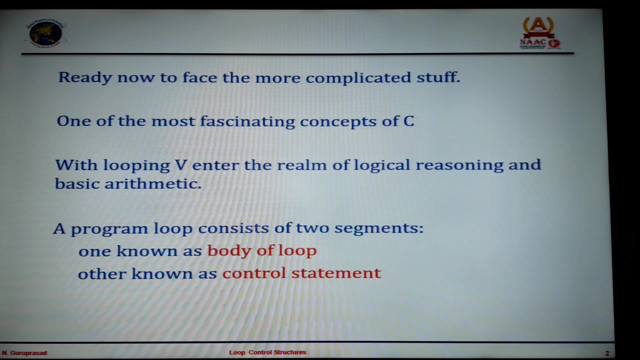 So basically, to solve, give solutions to these type of applications, we come out with a different type of control structures, what is called as loop control structures. What we have done in decision control structures is we executed the statement only once, when the condition is satisfied. But then in loop control structures, the fundamental difference is we are going to execute a certain set of statements as long as the condition is satisfied, And that is the advantage of loop control structures over decision control structures. 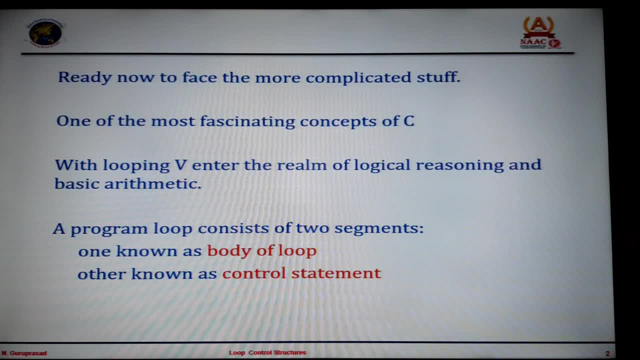 So it is considered to be one of the most fascinating concepts of C programming language, where we actually enter the realm of logical reasoning and basic arithmetic. And let me tell you, once we are accustomed with the entire concept of loop control structures, we can, we can expose ourselves to varieties of programs, which I will be doing it at the end of each subtopic of this particular topic. Now, basically, the 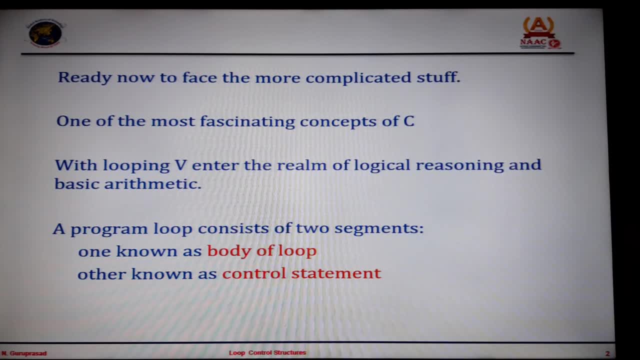 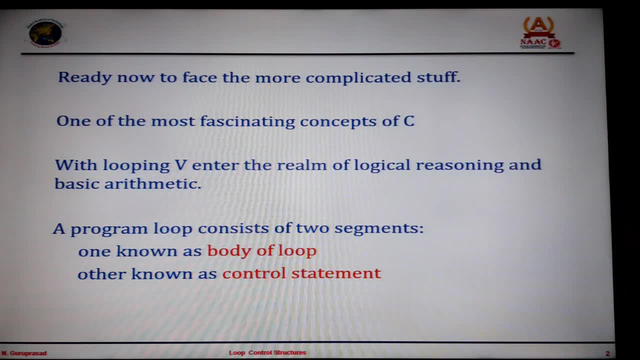 way from morning, say, for example, from morning 6 am to 6 pm, you are not very sure as to how many cups of coffee you drink. So these two types of approach is basically, or these two types of problems are actually tackled with what is called as loop control structures. Now any loop in a 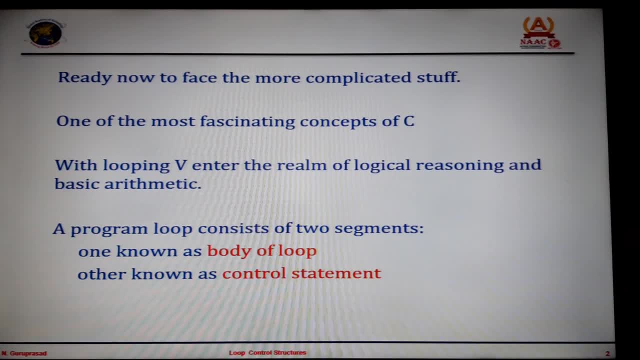 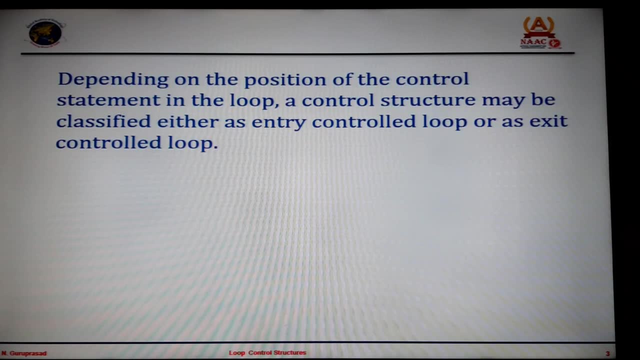 programming language consists of two segments: one, what we call it as a body of the loop, and other one is what we call it as a control statement. We will definitely look into both of these as we progress. Now, depending upon the position of the control statement in the loop, a control structure. 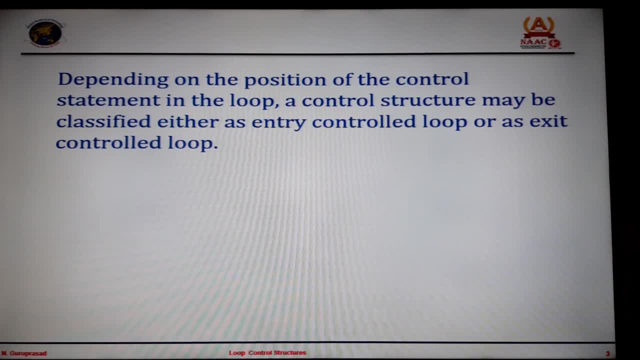 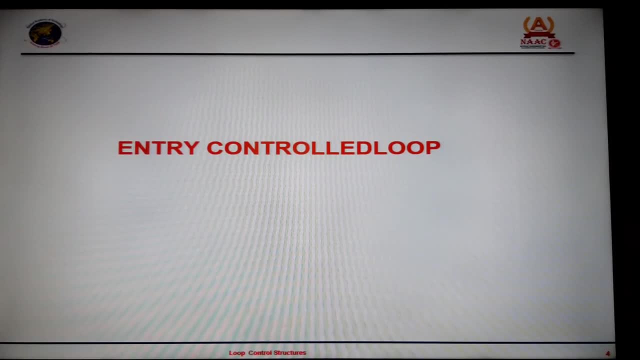 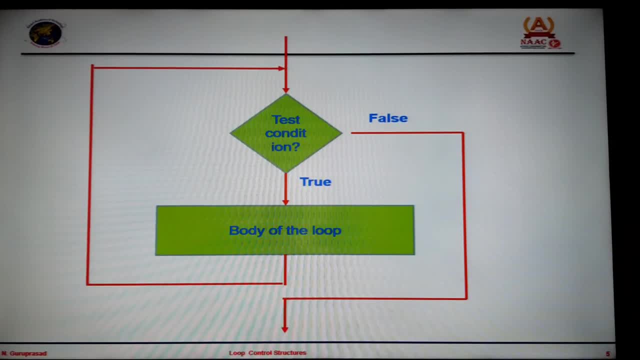 this is a simple flow chart how exactly your entry control loop looks like. You have a test condition first, and what happens is, if the condition is satisfied at the initial stages, the control of the operating system will go inside the body of the loop and then it will execute all. 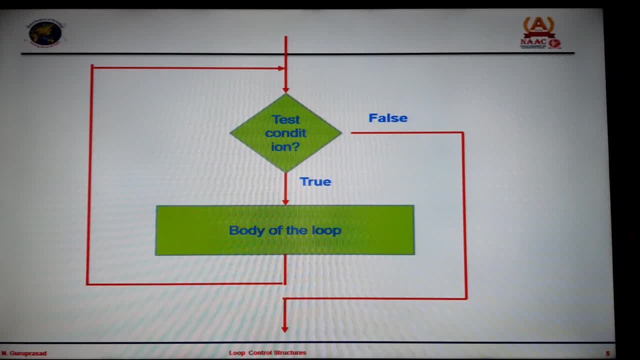 the statements which comes in the body of the loop. and once it executes all the statements, the control will go back to the test condition and check whether the condition is again true. If it is true it will go back to the process, but if it is false it will come out of the loop. Now the reason why. 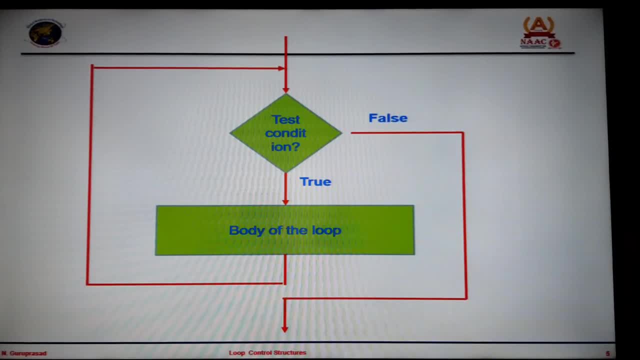 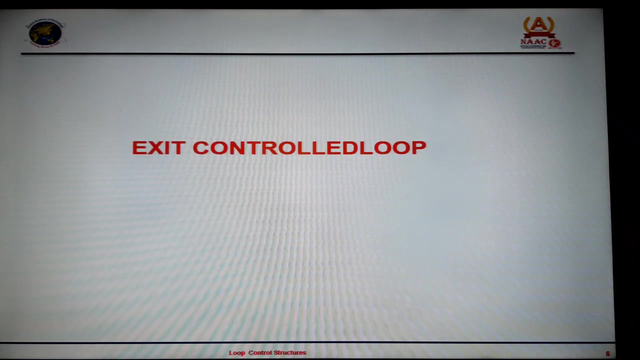 this is called as entry control loop is the condition is tested before the control of the operating system goes inside the body of the loop. That is the prime reason why it is called as entry control loop. On the other hand, if you look at the second type of loop, what is called as exit, 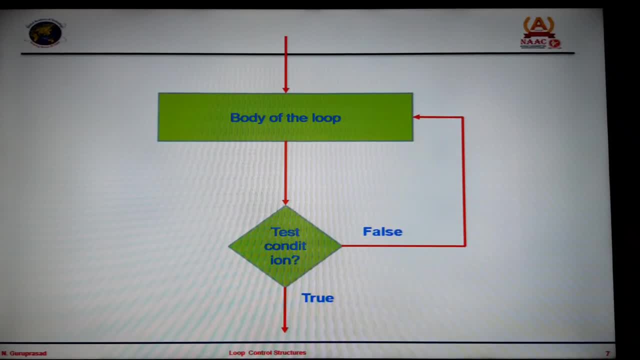 control loop. there is a slight change in how the flow chart looks like. In fact, if you look at the test condition, and in this the condition comes afterwards, As a matter of fact, the first thing is the body of the loop comes meaning first, all the statements in the body of the loop will be: 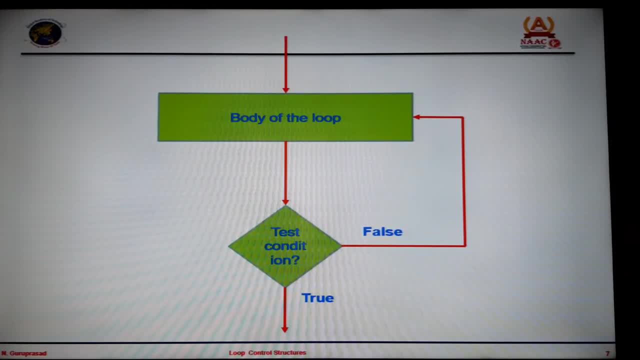 executed and then the condition will be checked. Now, if the test condition is true, then it will go back to the body of the loop. there is a small change in the type of error in the flow chart. So if the test condition is true, it will go back to the body of the loop, and if it is false, it will come out.